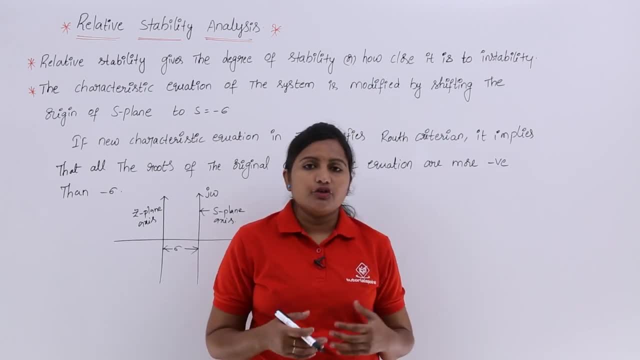 varying the parameters of the system then you may get the unstable system. For the same system you may get unstable condition if you are varying parameters. So root locus generally will give the better idea about this relative stability. but the to find out relative stability when characteristic equation is given that we will see in this. 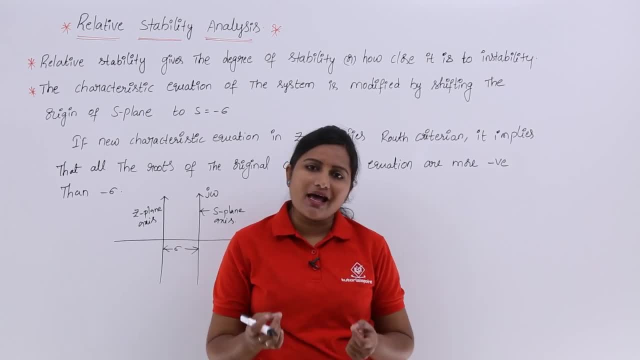 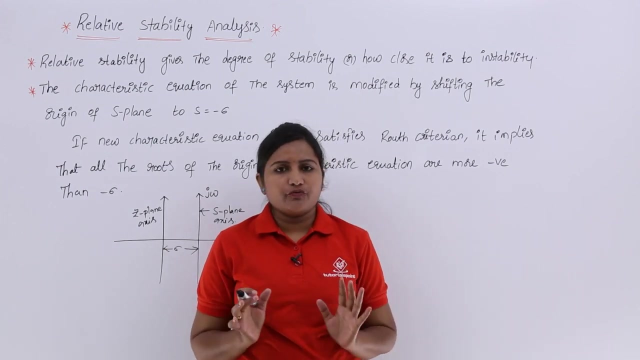 class. So generally you know that whenever you are having any characteristic equation describing a system, So generally, you are going to consider the route, hedge criteria, route array and from first column elements you are going to define whether system is stable or not. So same thing you are going to do here, but one point you need to follow. 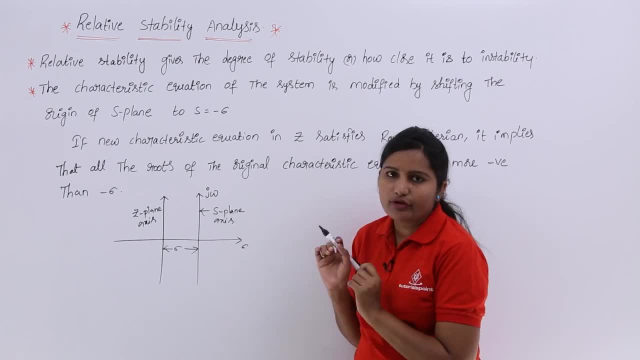 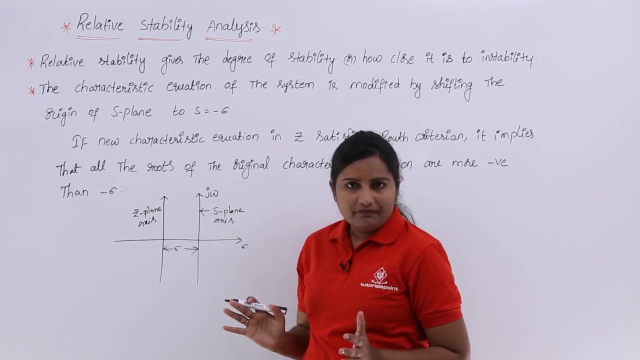 So generally, in diagrammatically, I will, I will give you an idea and I will give you two steps. according to the two steps, So we need to solve a problem in the next class. So this is the diagram indicating relative stability Generally, when you are considering, 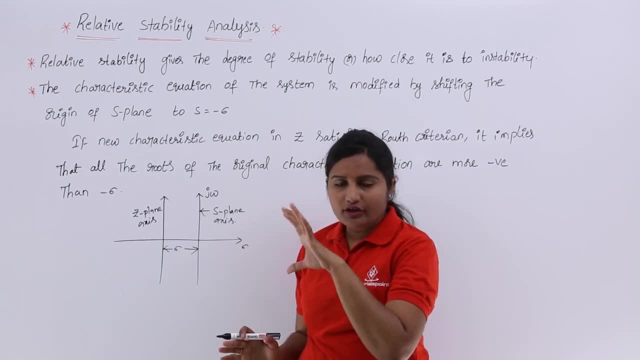 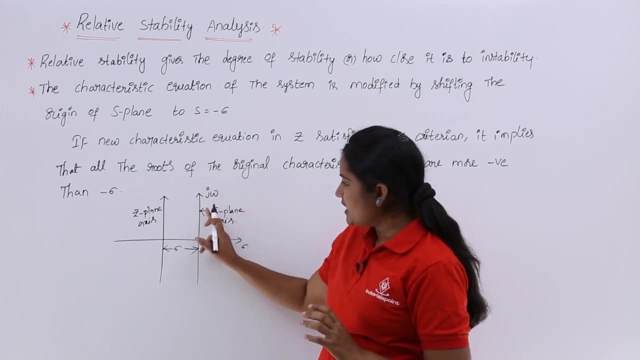 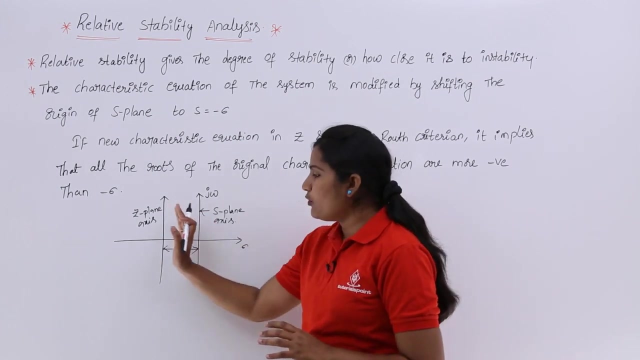 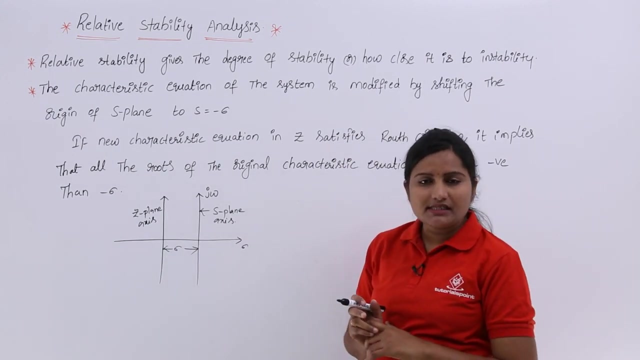 any S plane Or when you are considering any stability diagram, indicating diagram. So how you see it. So generally you will see S plane with real axis and j, omega axis, whatever the poles are there. if all poles on the left half of S plane, then we can say the system is stable. 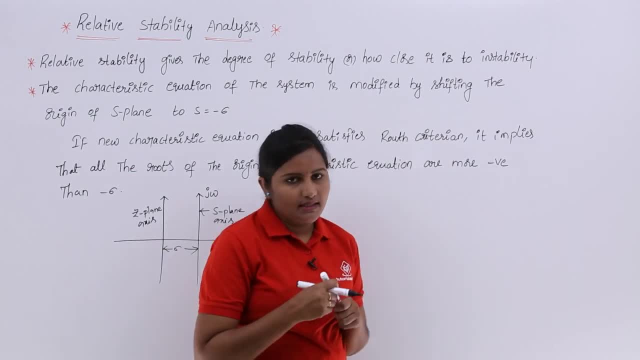 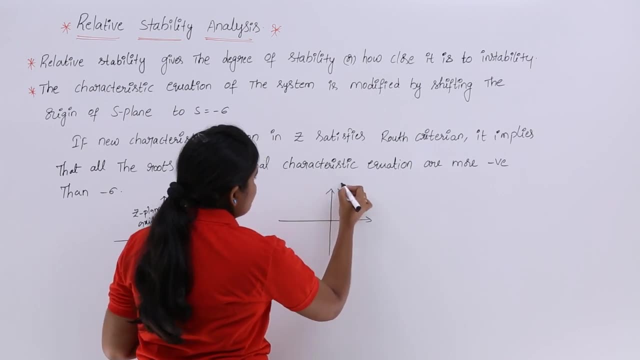 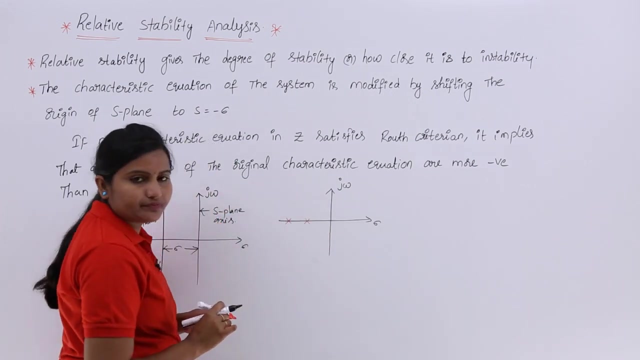 system. So that means. so here you can see, for example, typical 예 definition of Department of Sub생 il field. And here, if you consider base, I am having my system, pole 0, plot like this. So here I am having 2 poles like this. So 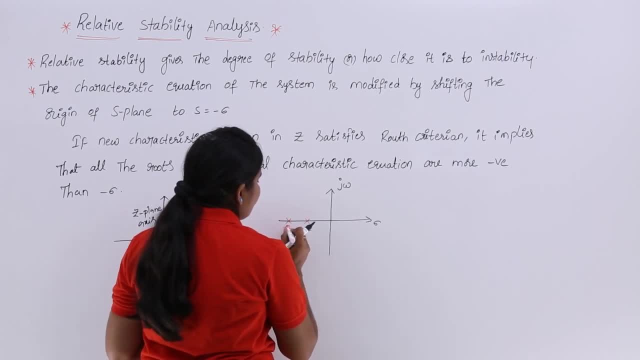 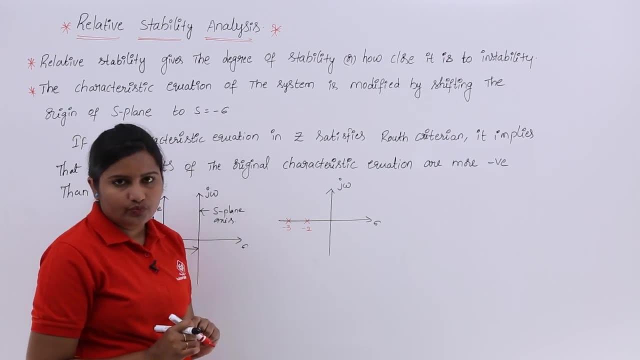 this pole at minus 2 and this pole at minus 3.. I am having 2 poles, So at minus 3 and minus 2.. So here, so in relative stability, first of all, this system is stable or not means So this is definitely a stable system. plot: This pole 0 plot is definitely a stable. 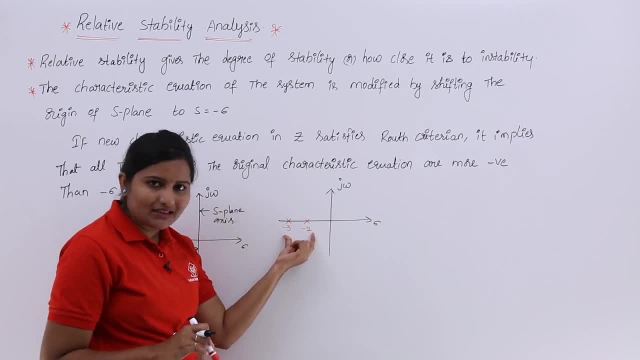 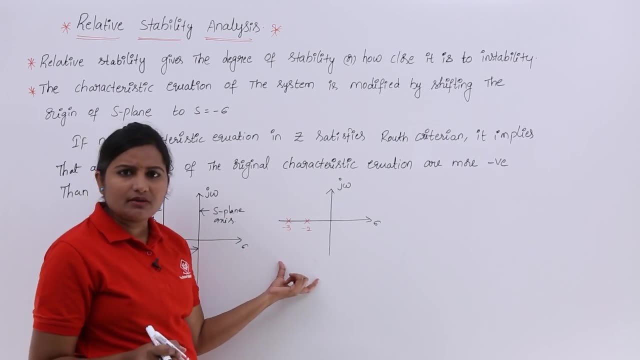 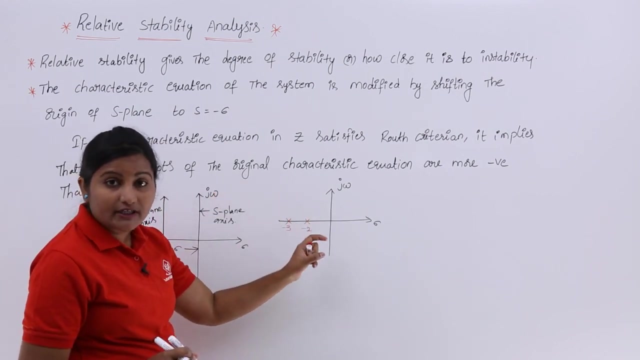 system plot. Why? Because whatever the poles we are having in this, all that poles are in the left half of S plane. So definitely we can say this is a stable system 1. So here to check how much stable it is, how much extent this is stable, how? 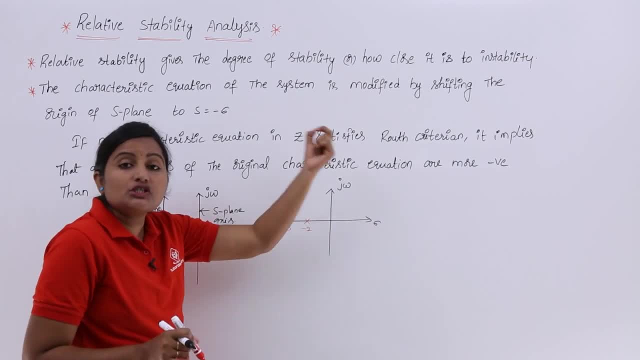 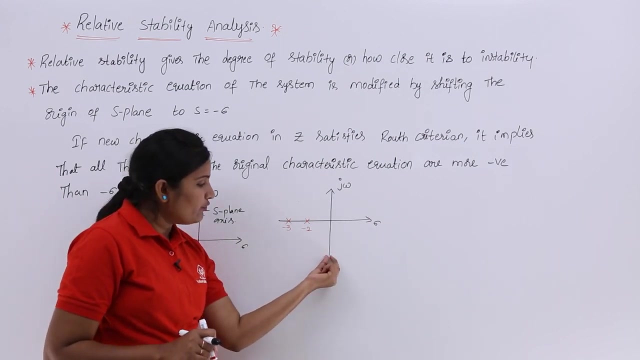 close to instable. this system is how much close to instability? that can be searched by using relative stability analysis. What we are doing in that analysis means So: we are changing this parameter, We are changing the origin, We are moving the source, We are 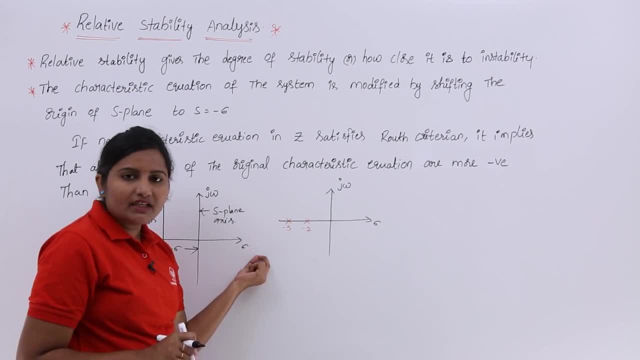 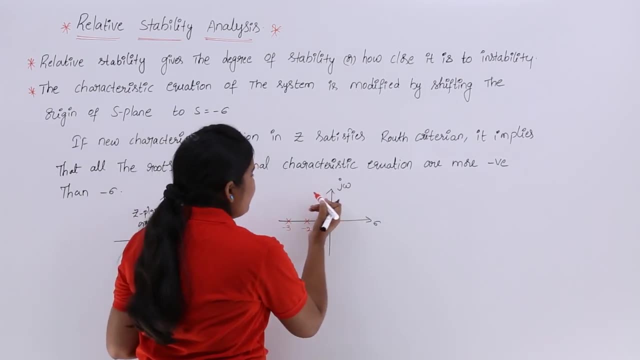 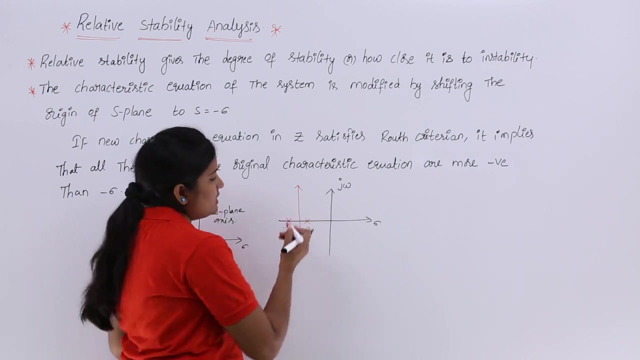 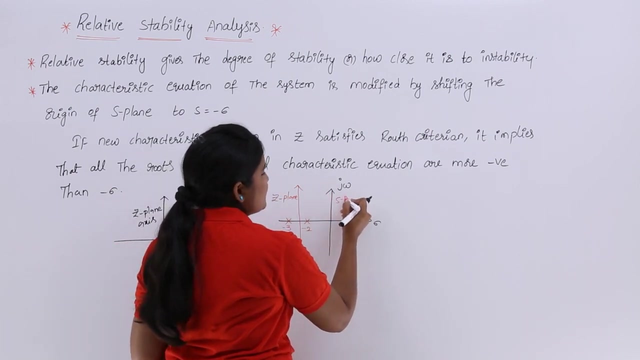 changing the origin, this side. We are moving this origin by a real value sigma, For example, I am moving my axis to here. So I am moving my axis to here like this. So this is my z plane axis, So this is my s plane Generally. S plane will contains imaginary axis in y. 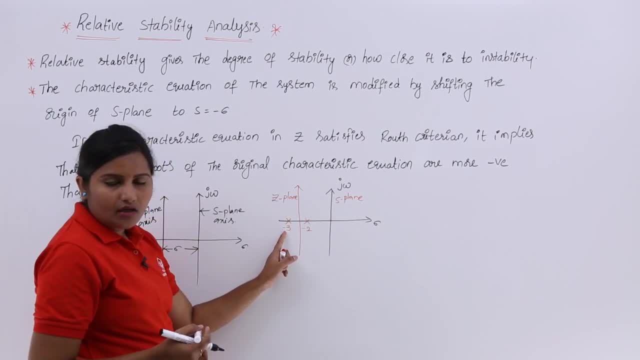 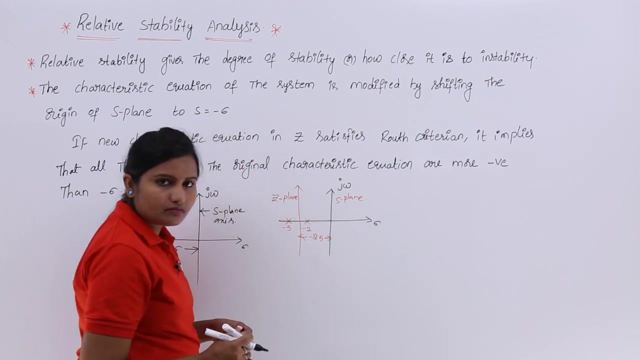 direction. So if you are moving, if you are moving, so here this j omega axis, if you are moving to some z plane, if you are moving your origin to some z plane which is in the distance of minus 2.5, for example, nothing but sigma. sigma is real value. 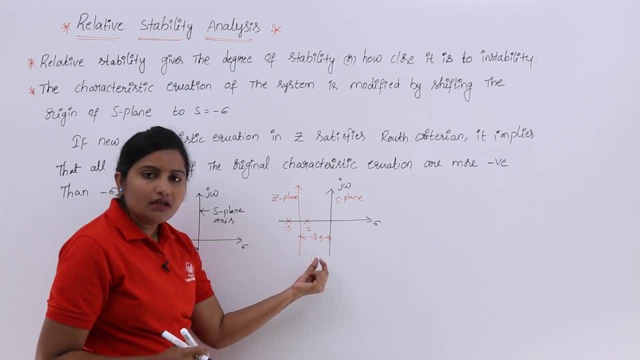 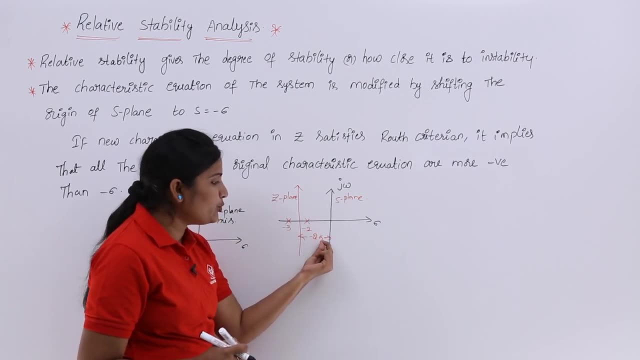 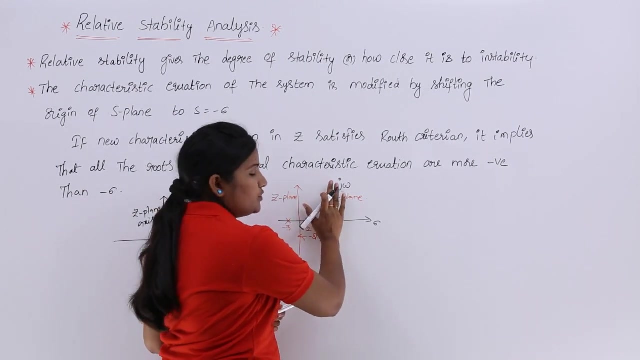 So 2.5 is a real value. So, for example, if you are moving your origin to a z plane which is in the distance of minus 2.5 from the actual axis, then you can see, then you just erase this axis in your mind. 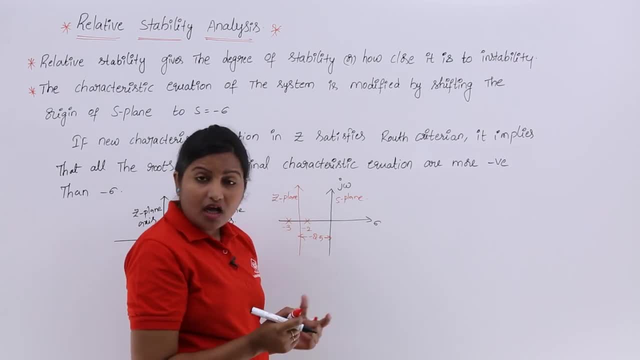 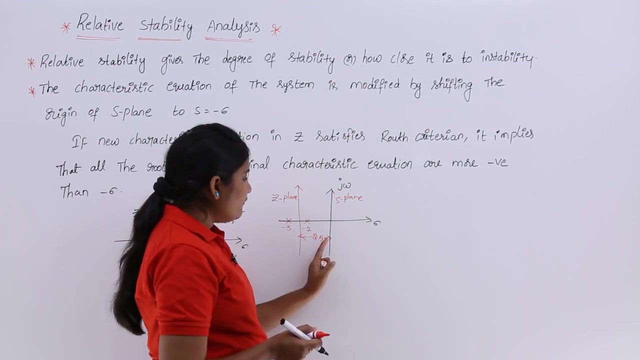 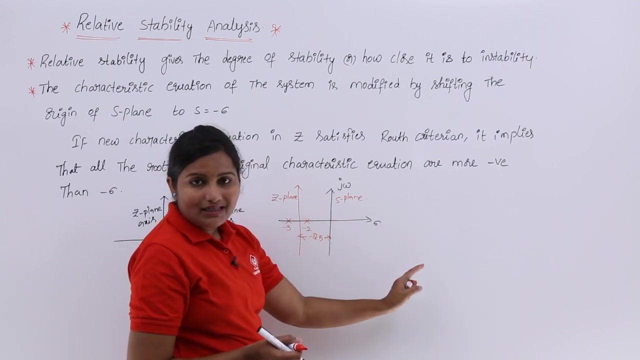 and go back. you just shift that to z plane. now the system is stable. now the system is stable means no, this system is unstable. now this system is said to be unstable system. so here, when you are moving this horizon to this z plane, one of the pole is in the right half of that horizon. 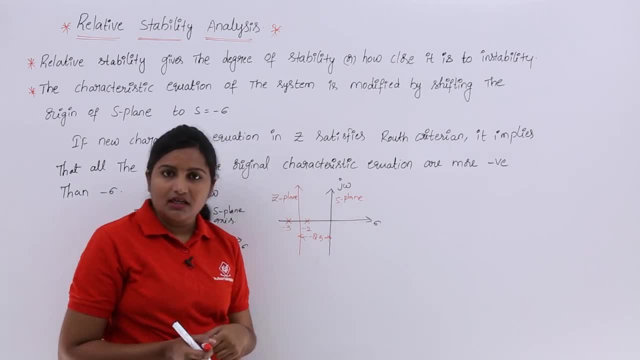 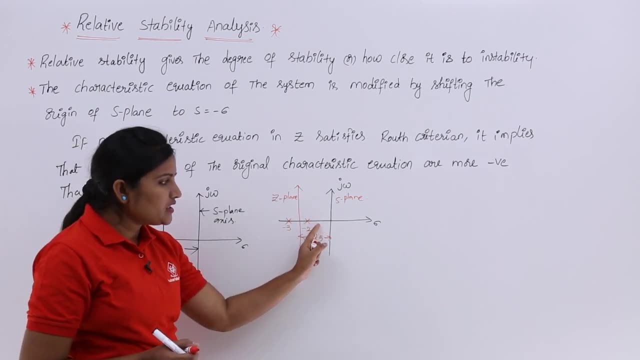 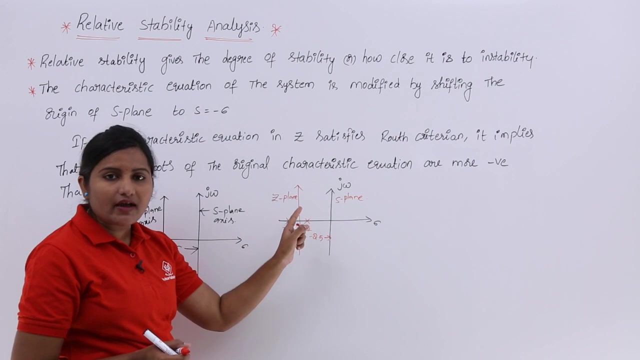 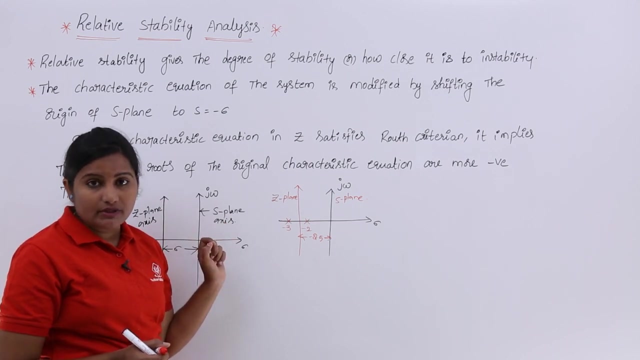 right half of that plane so we can say that is a unstable system. so before minus 2 only the system is relatively stable. otherwise if you are moving backward to this minus 2 then you can say that is relatively unstable system. you are going to get unstable system. that 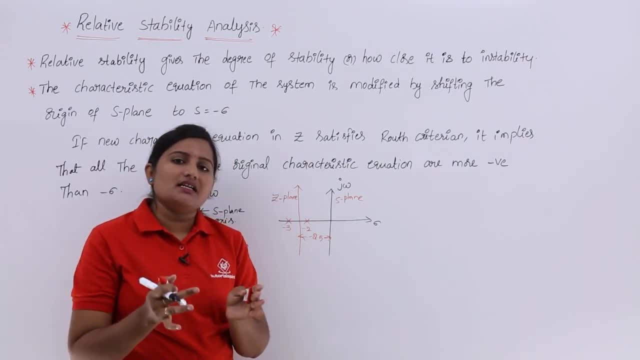 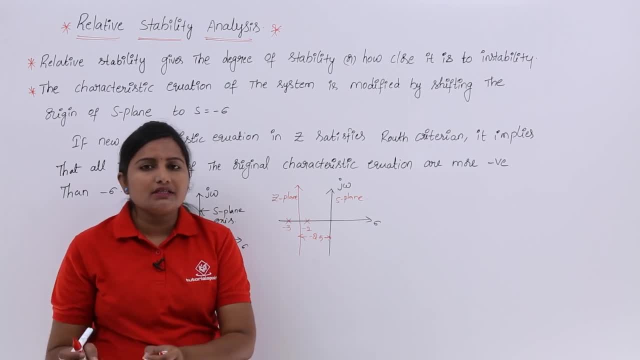 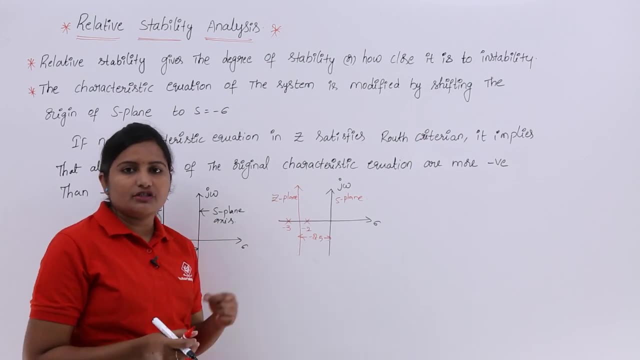 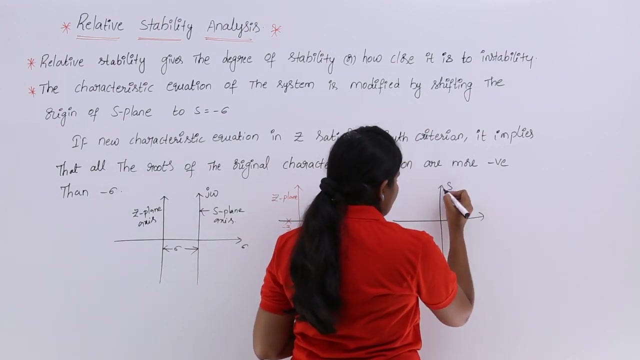 system is stable, how much extend this is stable, how much from which point we will get unstability, how close this system is to unstable So that we are going to discuss here, For example, same system I am going to consider: So this is S plane, and that means S plane. 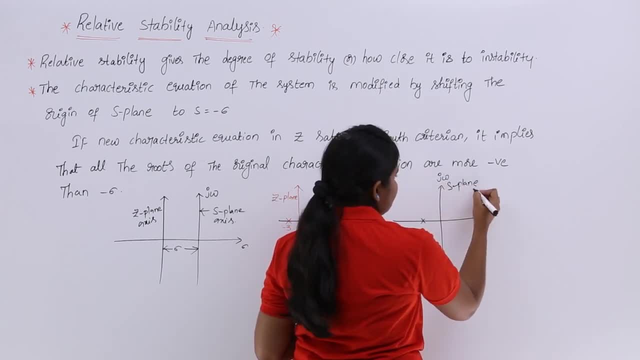 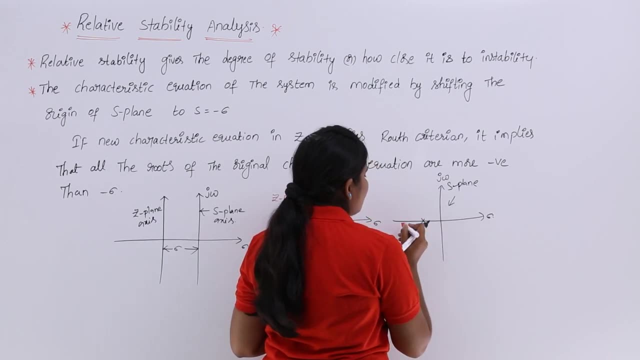 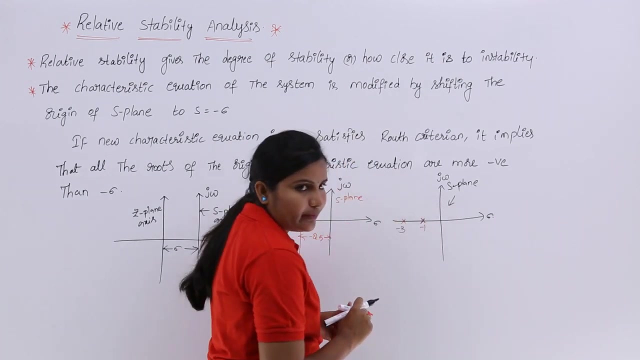 means this is j omega axis. totally this plane is S plane, So this is real axis. Here I am having a pole, So this is minus 1, and here I am having another pole, So that is minus 3, for example. Now this system is also a stable system. Why? Because all the poles 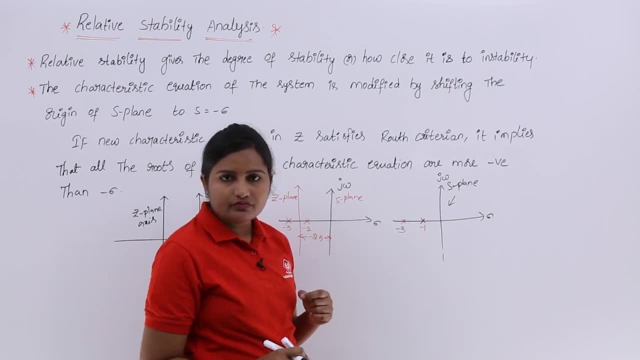 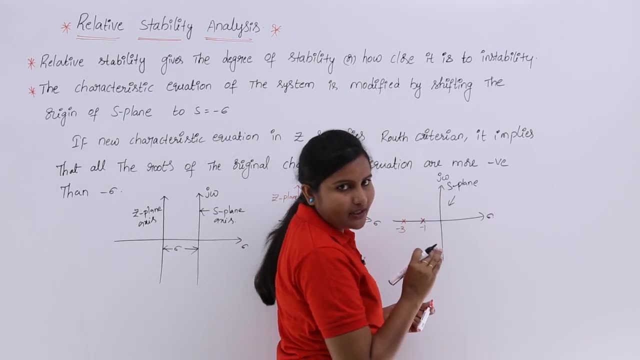 in the left half of S plane Now. so here you can see, this is a stable system. So this is a stable system where this is a stable system, So it is able to move whatever. so here it is a stable system, but in the left half of the S plane. So, for example, I am 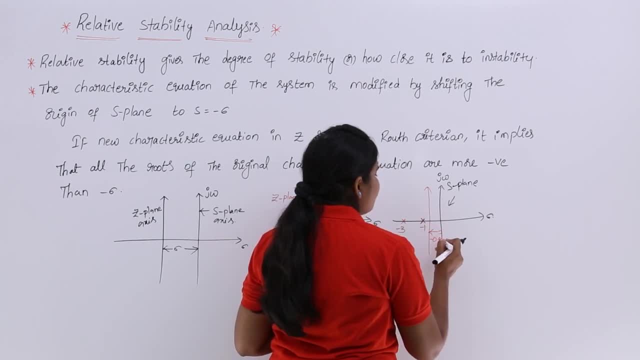 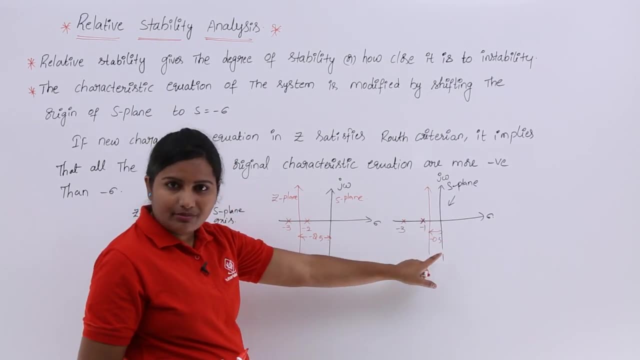 shifting to check the relative stability of the system. If I am shifting my origin to Z plane which is in the distance of minus 0.5.. Minus 0.5 is also a real value- I am shifting my origin with a sigma distance where my sigma is equivalent to minus 0.5.. Now what? 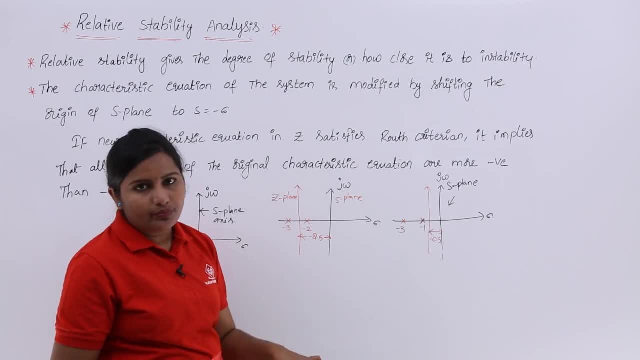 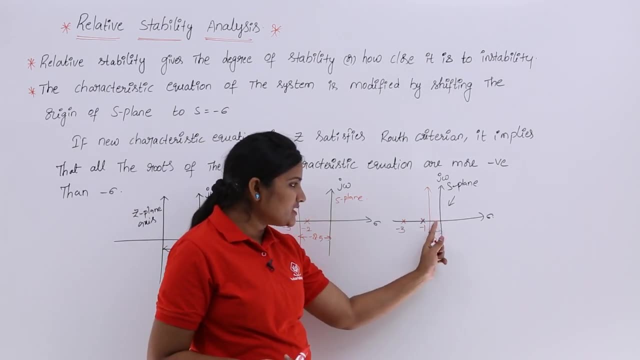 about this stability Now also, if I shift it slightly, that means I am shifting my origin with a sigma distance where my sigma is equivalent to minus 0.5.. Now, what about this stability Now also, if So your system is stable. Why? Because if you shifted this horizon to minus 0.5 also, 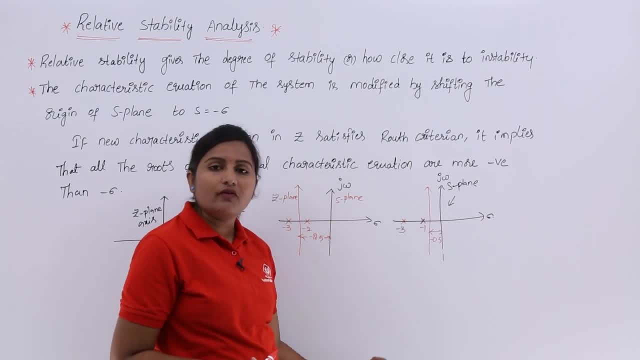 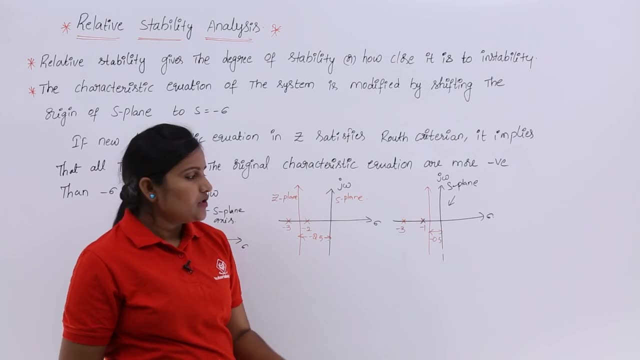 all the poles will lie in the left half of S plane or Z that plane only. So we can say the system is stable. So if you move further to minus 1, then your stability will decrease. If you are moving away or further from this imaginary axis, then your relative stability 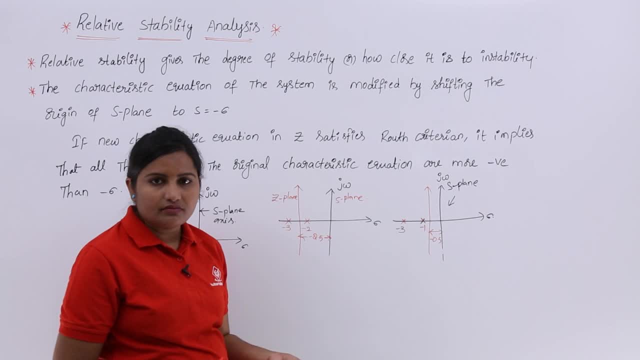 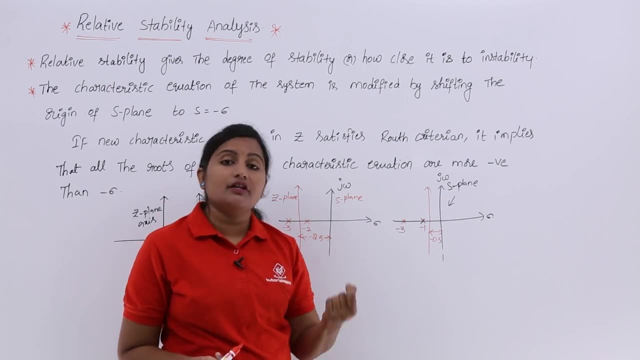 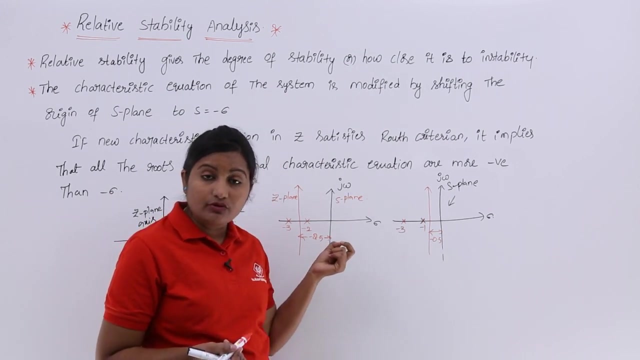 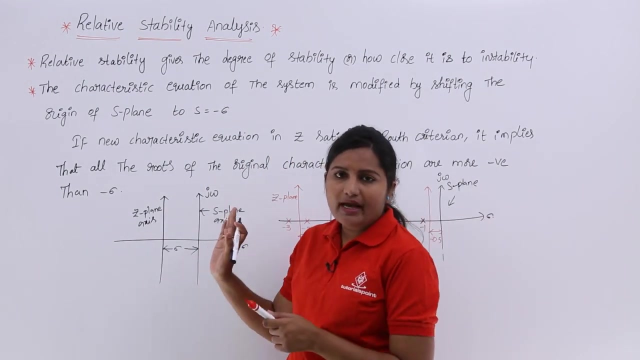 will increase. Your relative stability will increase. If you are moving further to j omega axis, then your relative stability will be increased. So here, if you are moving beyond this j omega axis, your relative stability will decrease. So now we can see this. what the diagram? So, by moving that origin to some distance, 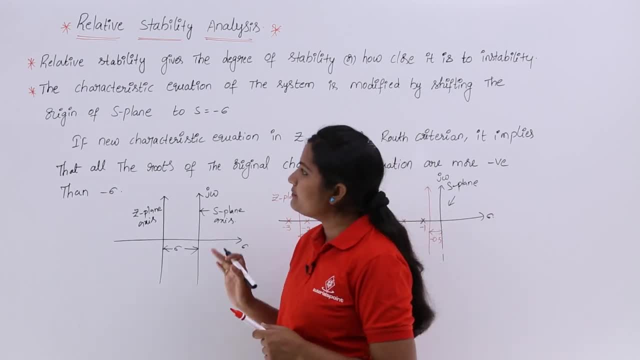 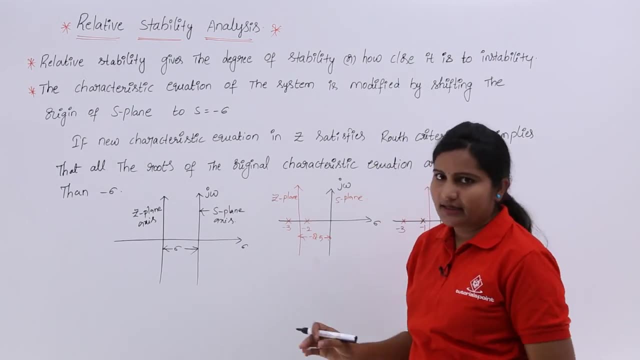 we are going to get the relative stability. So here the most important point is the characteristic equation. how, for example, if any characteristic equation is given, they are asking relative stability, Then how we can say: the relative stability means in the characteristic equation, in given characteristic equation we need to substitute the value, So here the given. 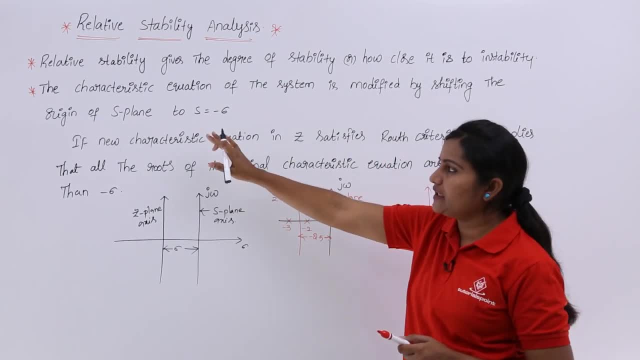 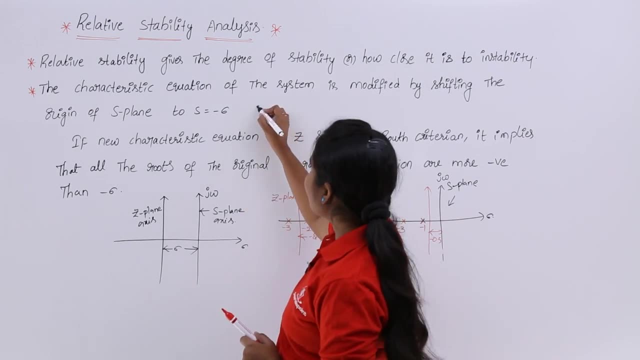 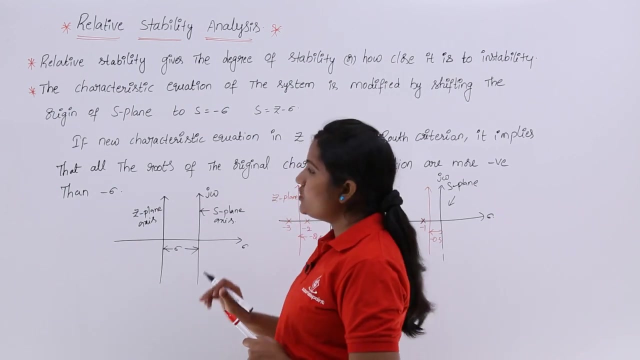 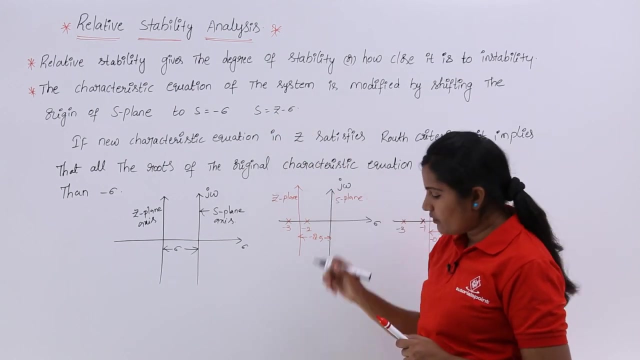 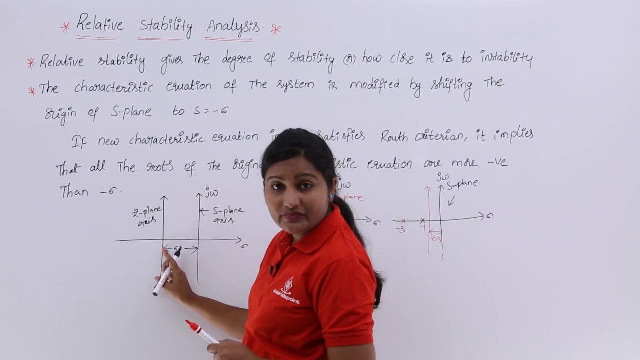 characteristic equation is modified by shifting the origin of S plane to: S is equivalent to minus sigma, or that means S is equivalent to Z minus sigma. as this is Z plane, you are shifting sigma distance, So you are using So why I am writing Z minus sigma? So you are moving S to minus sigma. this will become: 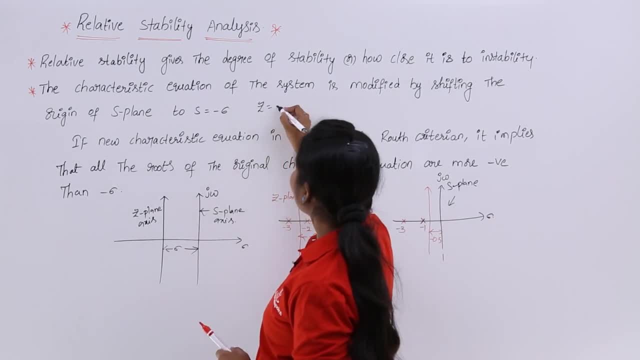 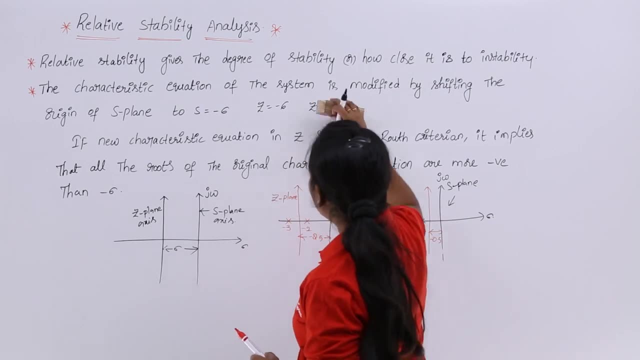 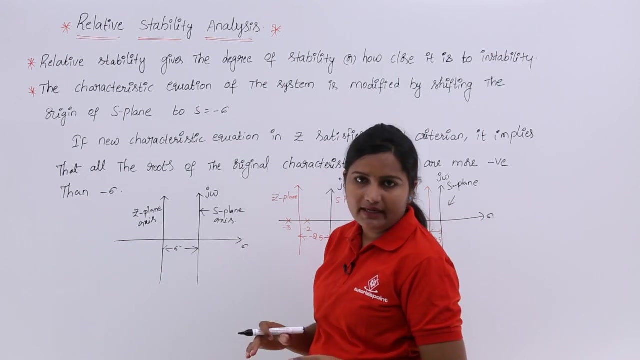 Z axis. So here my Z is equivalent to minus sigma. So you will get Z plus sigma. or you can write like this: You are moving minus sigma distance in S plane, or if you are moving minus sigma, it will become Z plus sigma. or you can write like this: this will become: 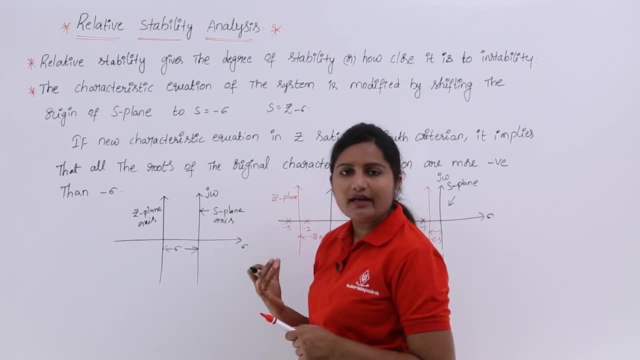 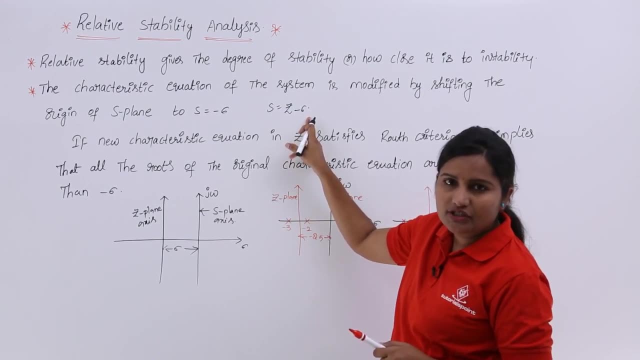 minus sigma or plus sigma, and in this case you will adjust the velocity quite well. Here, if you are showing Z and Q compared to your original-regular velocity of sigma, over here you are going to be using S. in this case you are Richardson weight as the relative rate that you are estimating. 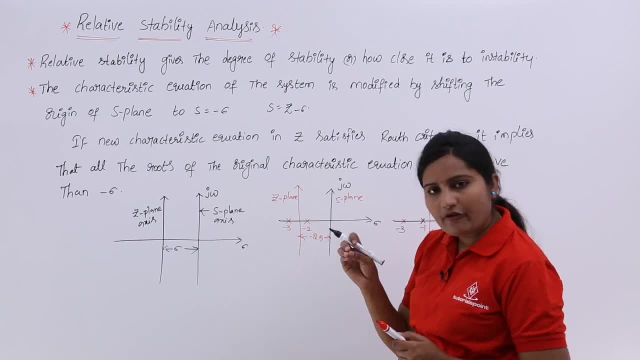 So it is very easy to make that testing: find the relative value�보기 to shift sigma, which in higher delta we have already seen that is not going to work. again to have projection terms of Z After substituting S is equivalent to Z minus sigma. you are going to calculate. 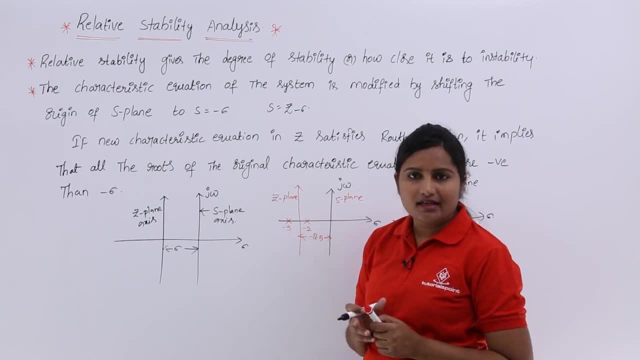 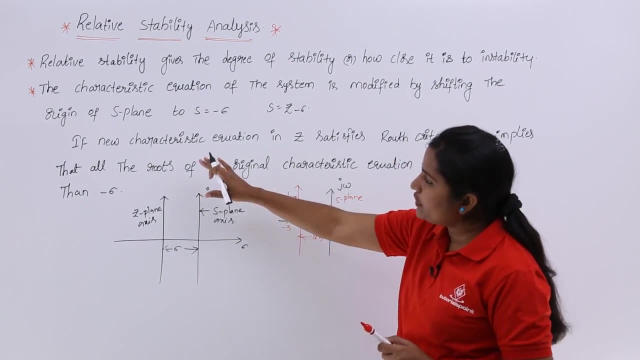 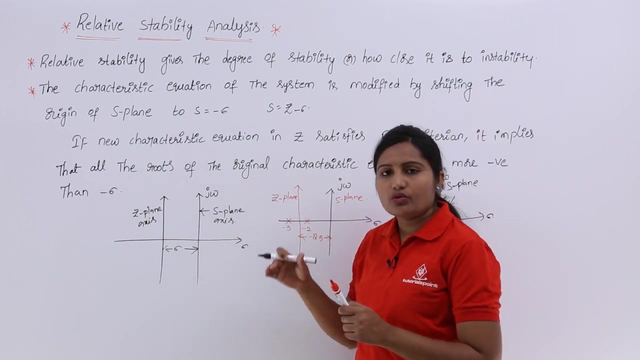 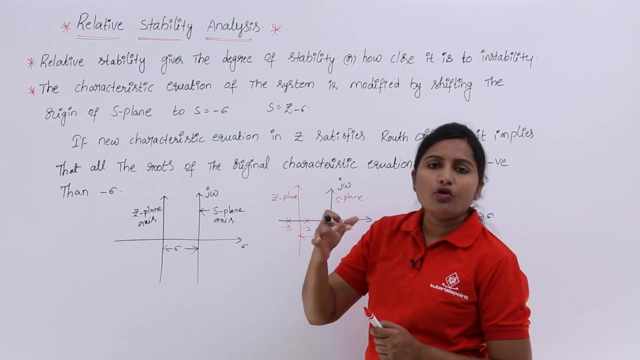 the simplified characteristic equation. For that characteristic equation we just calculate Routh array. After calculating Routh array, if new characteristic equation in Z satisfies the Routh criterion, it implies that all roots of that characteristic equation, all roots of the original characteristic equation, are more negative to this minus sigma. 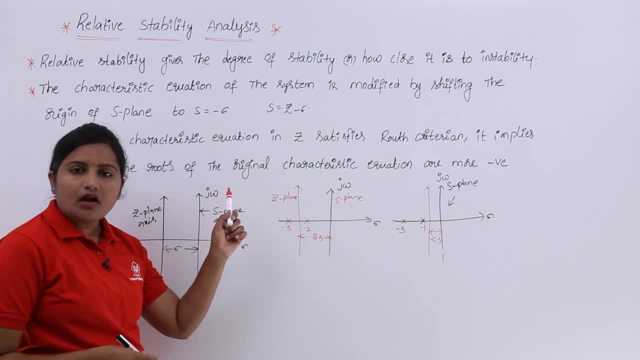 That what is the meaning of this point is. after substituting S is equivalent to Z minus sigma, the modified characteristic equation again satisfying the stability condition in Routh array. then we can say: all the roots of the original characteristic equation are said to be minus. 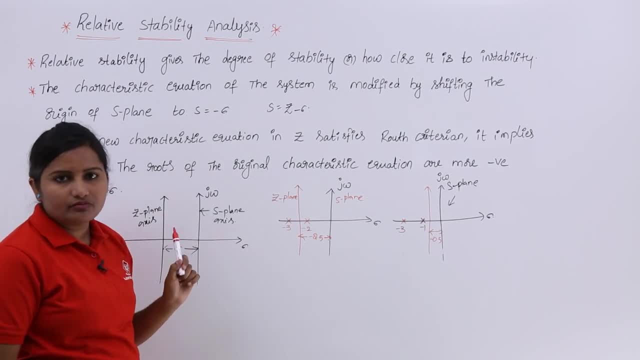 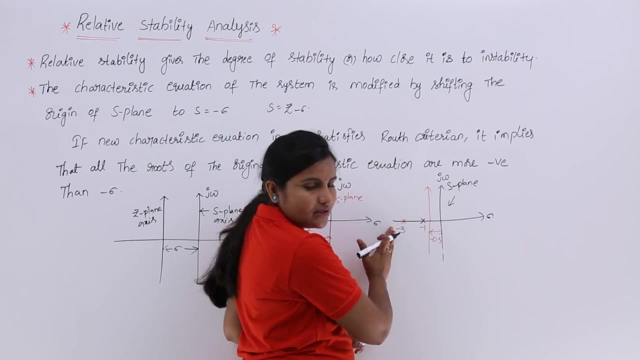 So all the roots of the original characteristic equation are considered to be more negative than our minus sigma value. That is nothing, but after changing. also, if you are getting stability condition, this is the meaning: all the roots of the original characteristic equation are more negative than our considered real value. Here the best example is this: 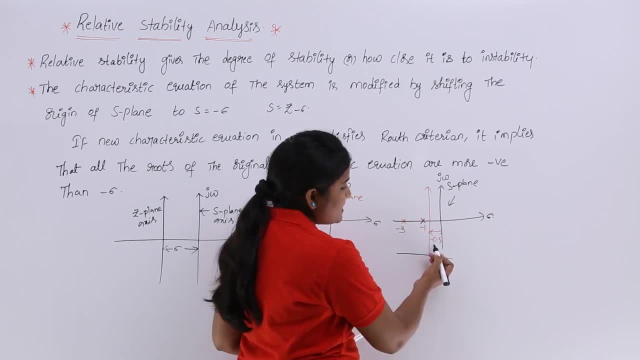 for that point. If you considered any real value and if you shifted that origin, you are getting the stable condition. So the stability condition of the root of the original characteristic equation is more than not. So you have to think about the stability. 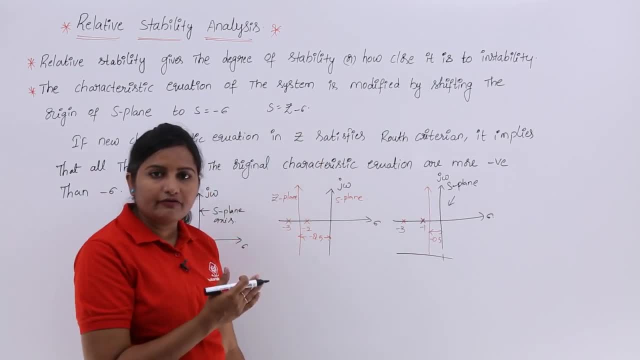 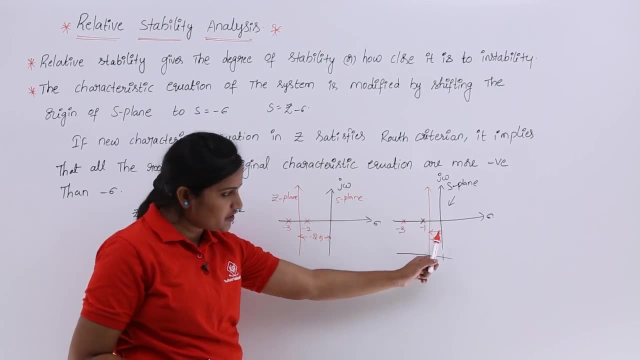 after shifting origin to that particular point. if you substituted in that characteristic equation again, if your system is stable, So here also system is stable after shifting also, then in this condition we can say all the roots of the actual characteristic equation are more negative than the considered root. Here you can see minus 3, minus 1 or more negative than